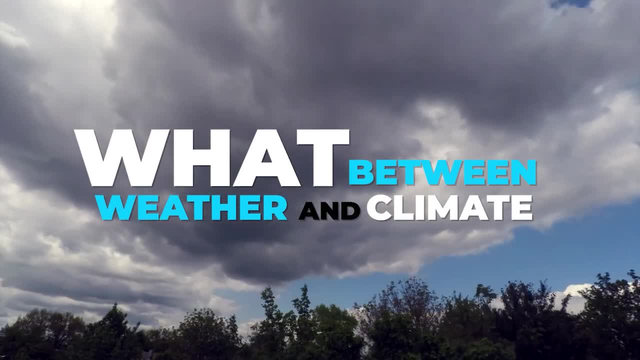 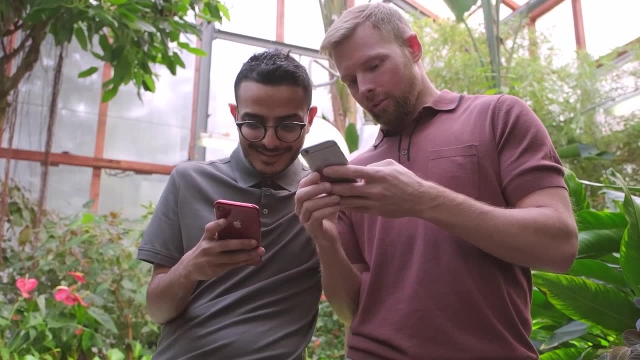 the question: what is the difference between weather and climate? By the way, if you enjoy content like this, don't forget to hit the like button, subscribe to the channel if you're new and turn on notifications so that you never miss a new video. Let's get started. The terms weather: 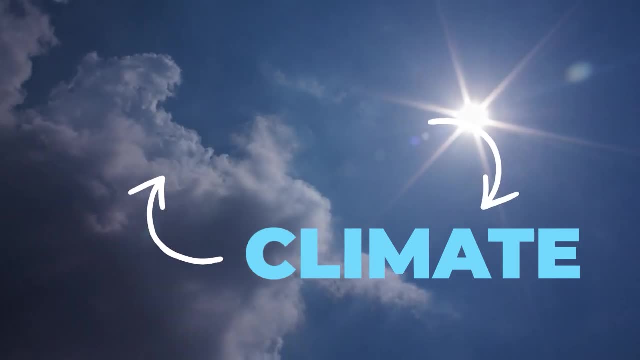 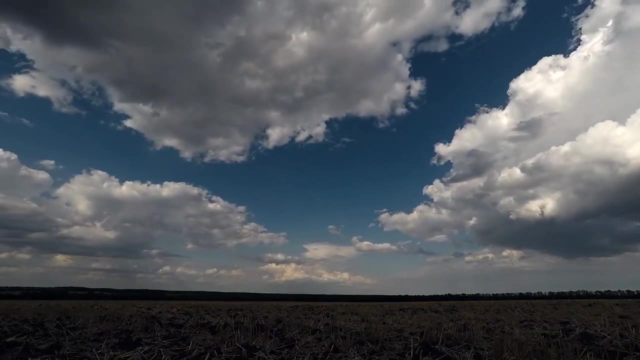 and climate are used interchangeably, with many believing that they're one and the same. However, the two are incredibly distinct from each other, which is why it's important to learn their key differences. Weather refers to the short-term conditions of the Earth's atmosphere. 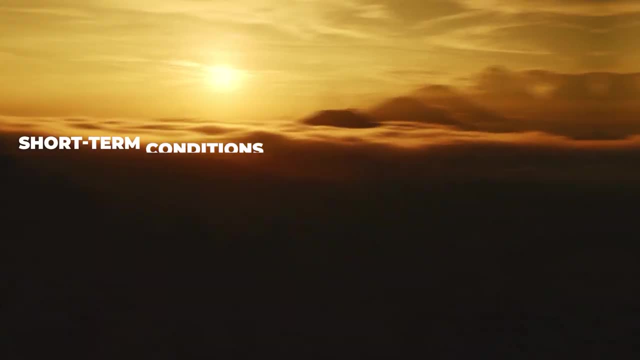 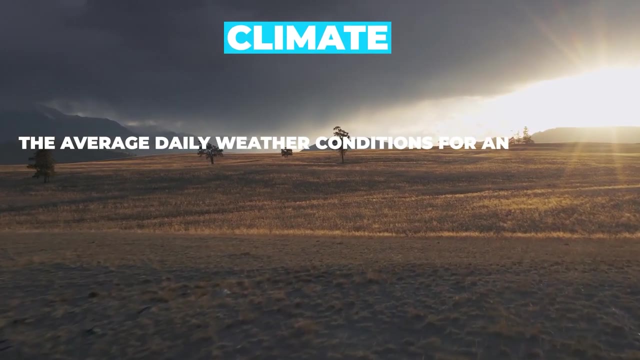 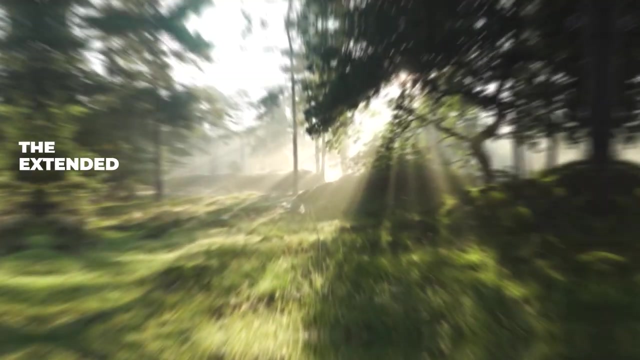 which is basically what you see outside on any given day. So heavy rains tomorrow and snowfall on the weekend are both examples of weather. On the other hand, climate means the average daily weather conditions for an extended period of time at a particular location. More specifically, the averages of precipitation, temperature, humidity. 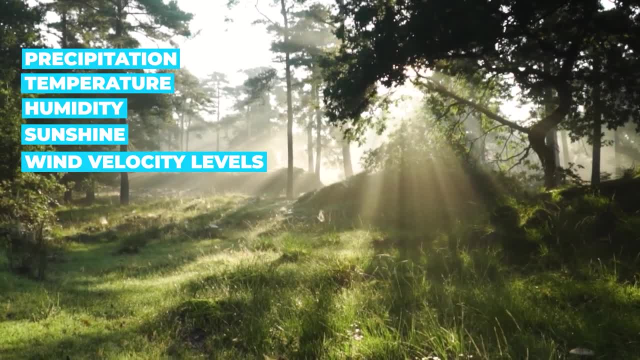 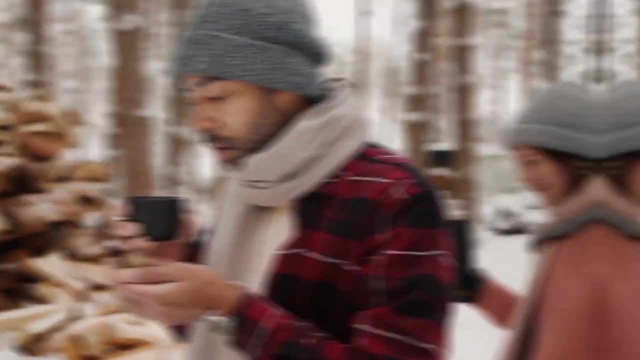 sunshine and wind velocity levels are used to determine the climate of a place. Other events like fog, storms and frost are also taken into consideration. For instance, due to the climate of Massachusetts, the state experiences hot and humid weather in the summer. 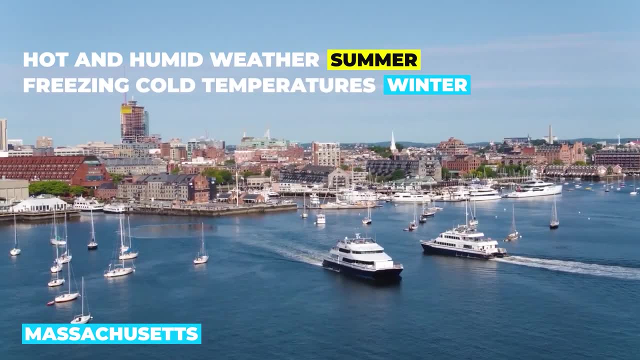 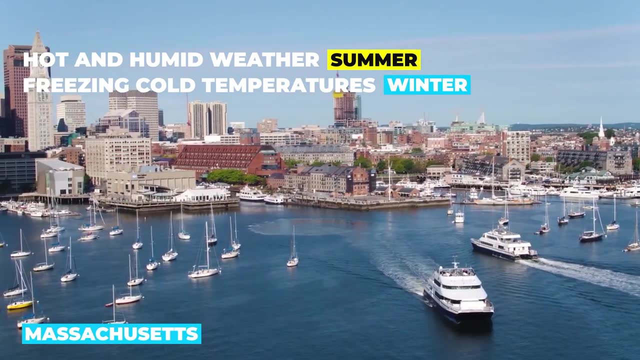 with freezing cold temperatures in the winter. It's important to note that the weather changes constantly. It can be rainy in the morning and scorching hot in the afternoon. However, the climate is the average of this weather over a prolonged period of time. 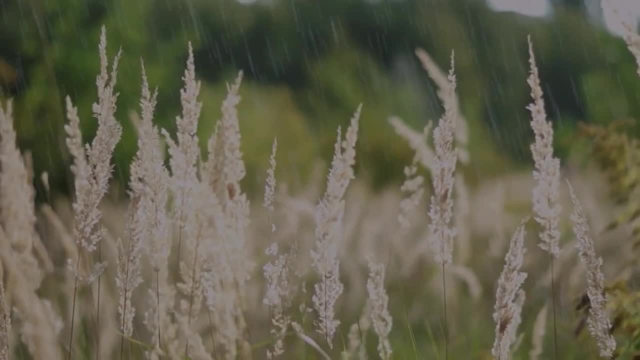 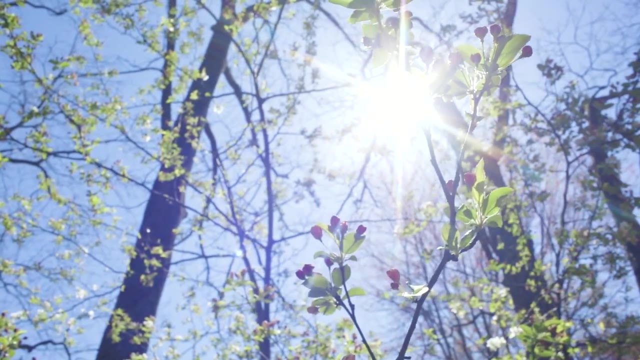 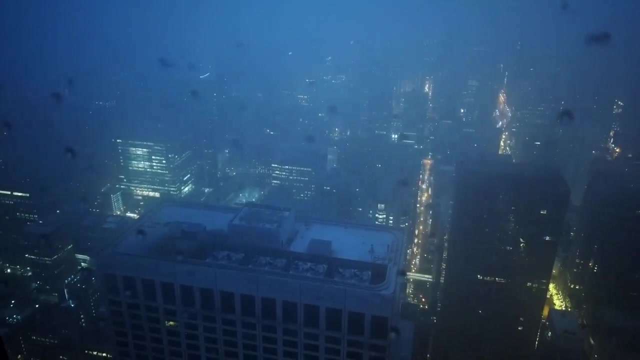 So what does weather consist of? In many places, weather changes hour to hour, day to day and season to season. Its components include events like sunshine, hail, blizzards, thunderstorms and heat waves. Some of these can become very devastating for the area they affect. For instance, experts estimate that approximately 400 people die from blizzards each year in the United States alone. Meanwhile, Super Typhoon Goni and Typhoon Vamco, which both hit the Philippines in late 2020, affected around 3 million people, with a death toll that stood at more than 100. 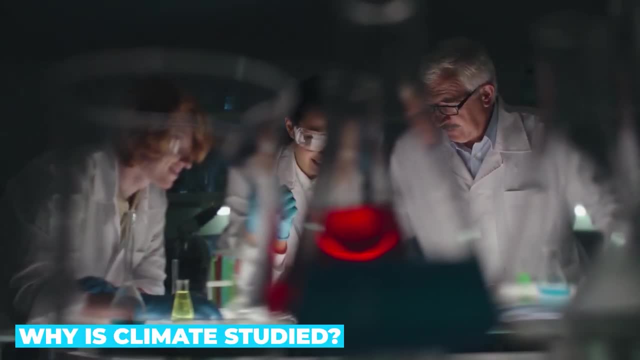 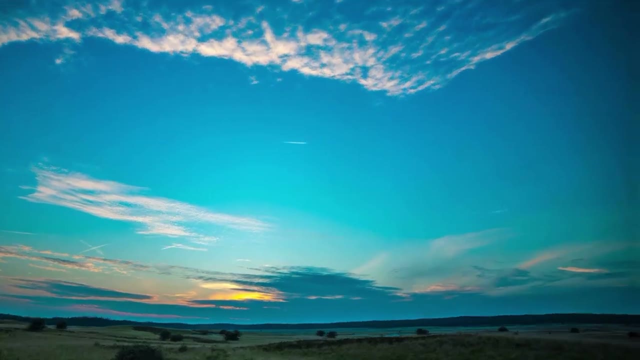 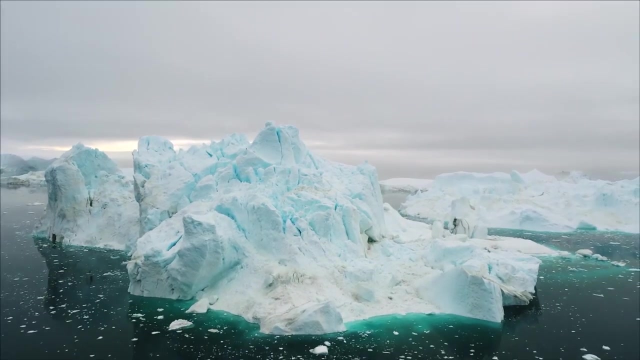 Given all these facts, you might be wondering why exactly climate is studied. After all, isn't it simply the average of all weather events experienced by a specific place? Well, it's more than that. Climate and the way it changes affect the entire world. For example,